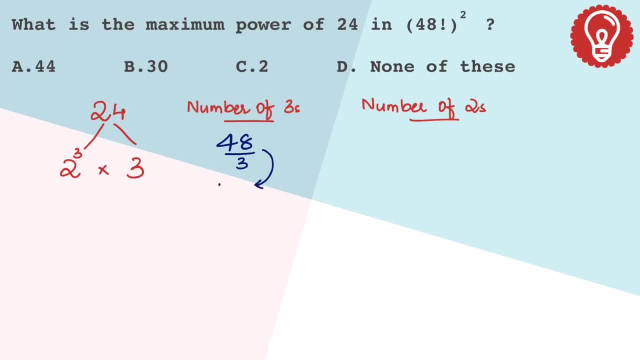 by 3, the first quotient is 16.. 16 when divided by 3 is 5.. 5 when divided by 3 is 1.. The sum of all the quotients is 22.. And 48 when divided by 2, the first quotient 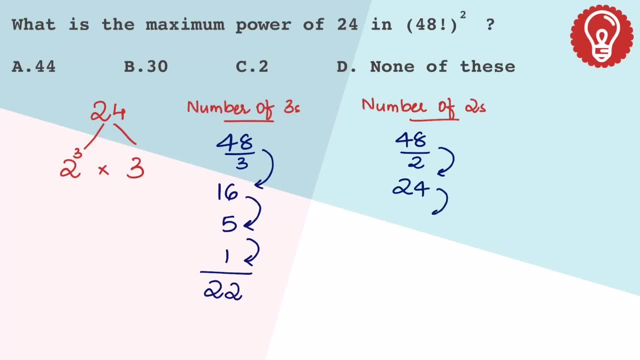 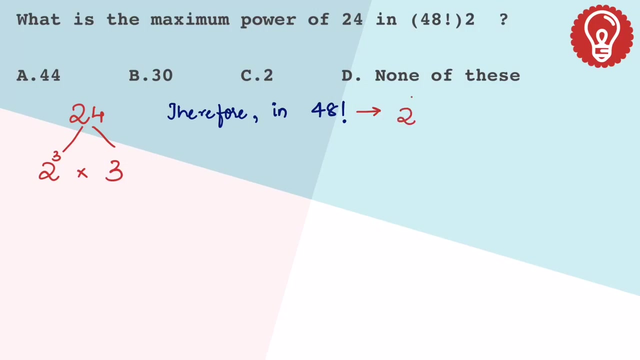 is 24.. 24 divided by 2 is 12.. 12 divided by 2 is 6.. And 6 divided by 2 is 3.. 3 divided by 2 is 1.. Now, sum of all the quotients is 46. Now, in 48, factorial 2s are 46 in number. 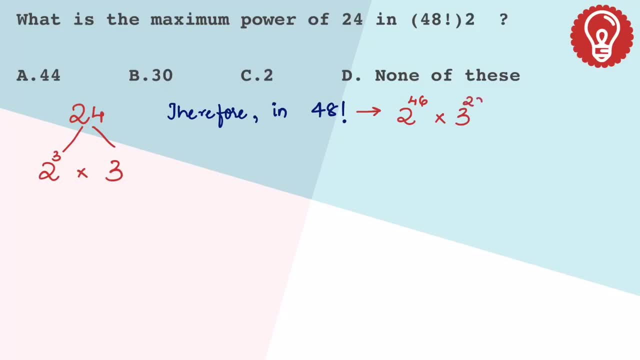 and 3s are 22 in number, Then obviously in 48 factorial whole square, 2s will be 92 in number and 3s are 44.. Let's focus on 2 power 92, because 2s should be represented in terms of 2 cube and 3s in terms of 3 power. 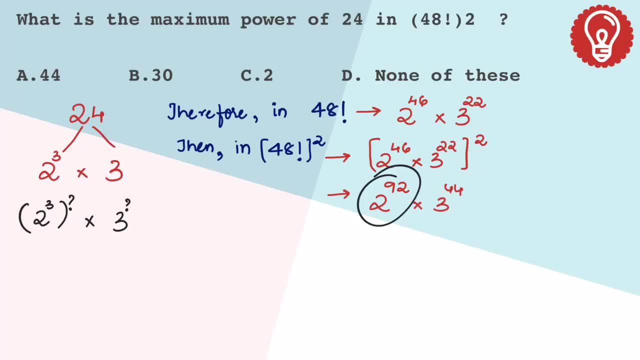 1.. So 92 is not divisible by 3.. Therefore the closest number to 92 which is divisible by 3 is 90. So let's write 92 as 2 power 90 and 2 power 2.. And 3 power 4 is sorry, 44. 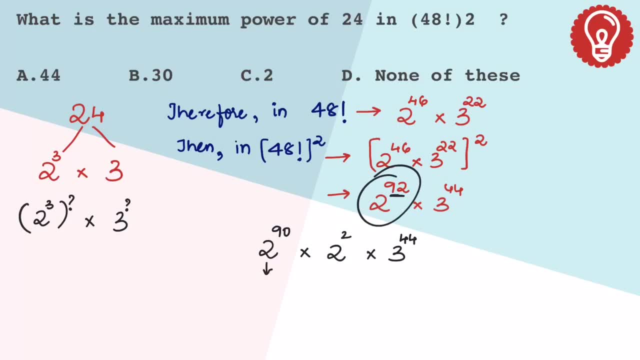 is as such. Let's express this in terms of 2 cube. 2 cube into 30 and the number of 3s are 44. And 2 square is the same. We know a combination of a 2 cube and a 3 will give us a 24.. So 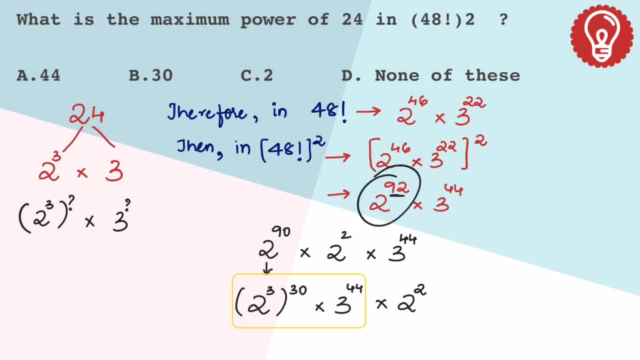 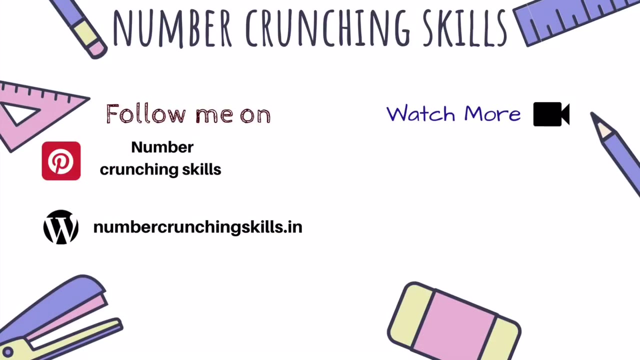 the focus is only on that. 2 cubes are 30 and 3s are 44 in number. We know that the smallest power is the answer. Therefore, 30 is the correct answer. The inside of the answer will be 43. So the answer will be in the underlying matrix. Now you remember that 1 cube is equal to the left side of the answer And 1 square is equal to the right side of the answer. The answer is right here. Here 3 square. Here, 3 square. The answer is right here. 3 square is equal to 1 square.